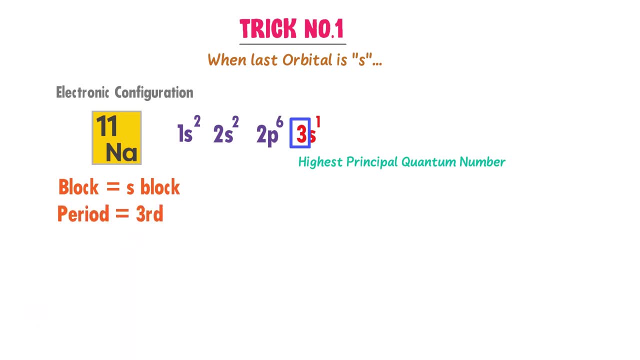 principal quantum number is 3.. So the period of sodium is third. There is only one electron in the last s orbital, So the group number of sodium is first. Also remember that if the last orbital is s, or p subgroup will always be a. The last orbital of sodium is s, So its subgroup is a. 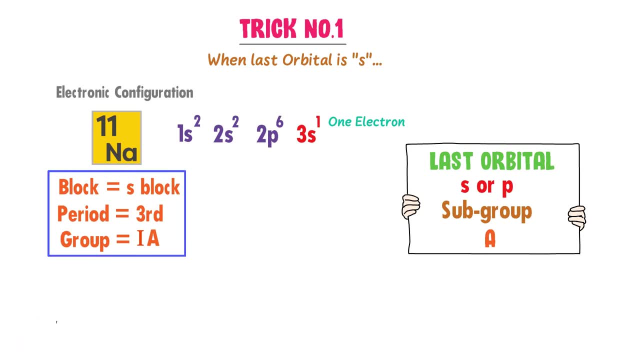 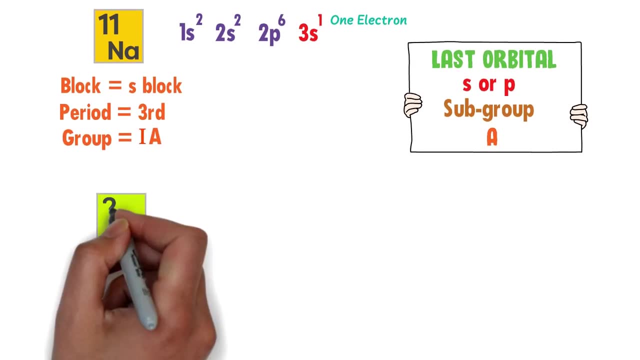 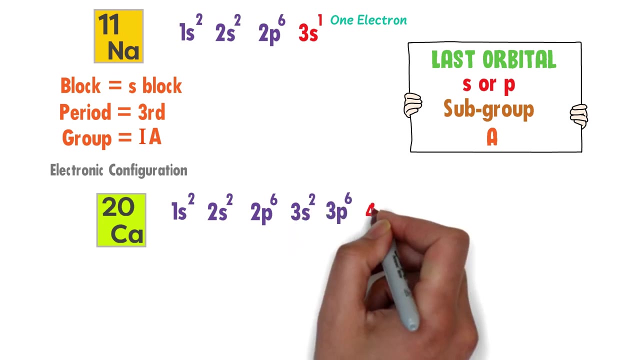 Hence sodium is s block element. It is present in the third period and first a group. Secondly, consider calcium, and its atomic number is 20.. The electronic configuration of calcium is 1s2, 2s2, 2p6, 3s2, 3p6 and 4s2.. If I add all these electrons I get 20 electrons Hence. 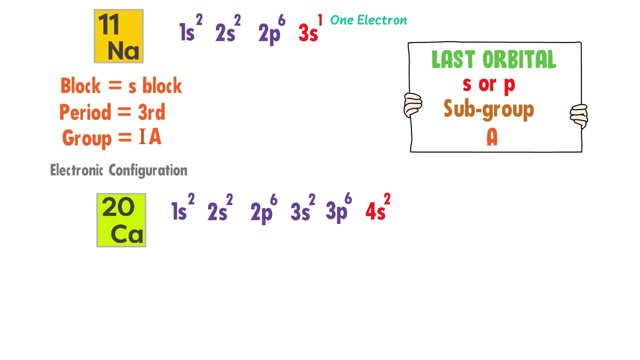 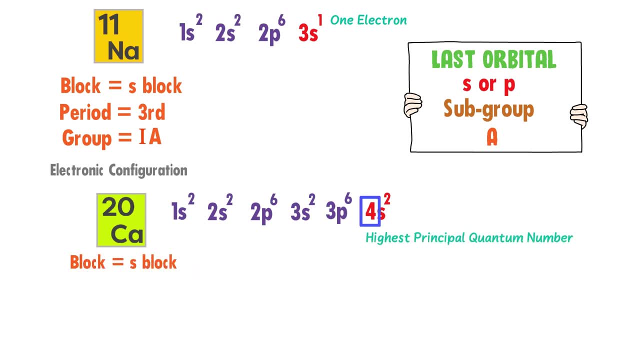 element. The highest principal quantum number of calcium is 4.. So the period of calcium is fourth. There are two electrons in the last s orbital, So the group number of calcium is second. We know that if the electrons of an element stay either in s or p orbital, its subgroup is always a. 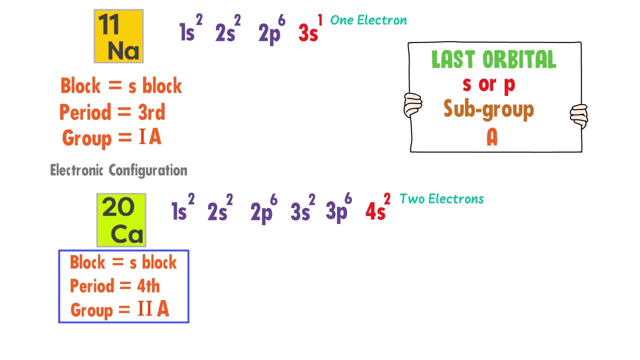 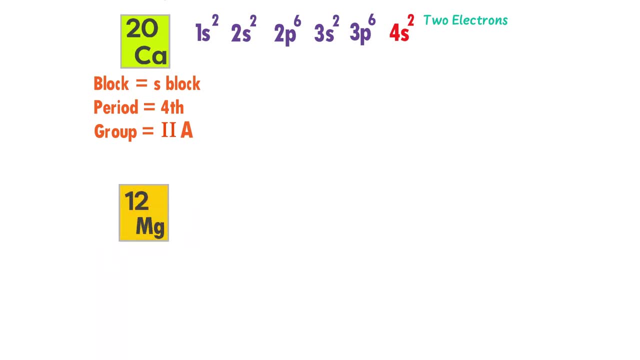 Thus calcium is s block element. It is present in the fourth period. Secondly, consider magnesium, and its atomic number is 12.. The electronic configuration of magnesium is 1s2, 2s2, 2p6 and 3s2.. If I add these electrons, I get 12 electrons Hence. 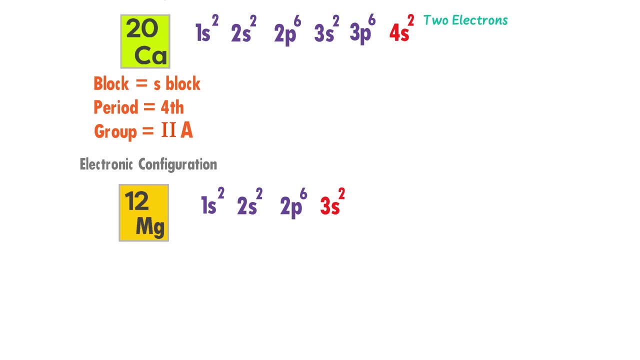 I have successfully configured the electrons of magnesium Here. the last orbital of magnesium is s, So magnesium is s block element. The highest principal quantum number of magnesium is 3.. So its period is third. There are two electrons in the s orbital of magnesium, So the group number of magnesium is second, The last. 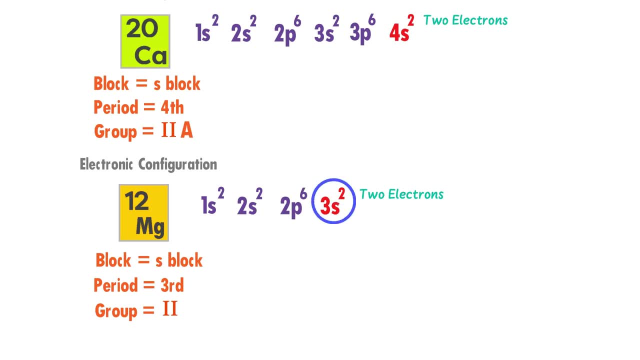 orbital of magnesium is s, So the subgroup of magnesium is a. Thus magnesium is s block element. It is present in the third period and second a group. Now let me teach you about the second trick. when the last orbital is p, 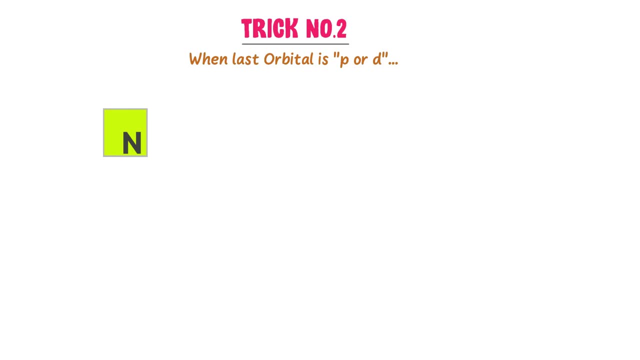 PRD. For example, consider nitrogen, and its atomic number is 7.. The electronic configuration of nitrogen is 1s2,, 2s2, and 2p3.. The last electron of nitrogen is in the p orbital, so the block of nitrogen is p. The highest principal quantum number is 2, so the period 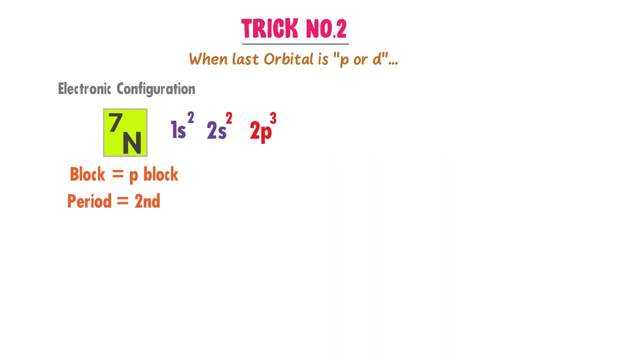 of nitrogen is second. Now listen carefully When the last orbital is PRD. always add the electrons in p and s orbital to get a group number. For example, in this p orbital there are 3 electrons and there are 2 electrons in this s orbital. 3 plus 2 is equal to 5.. 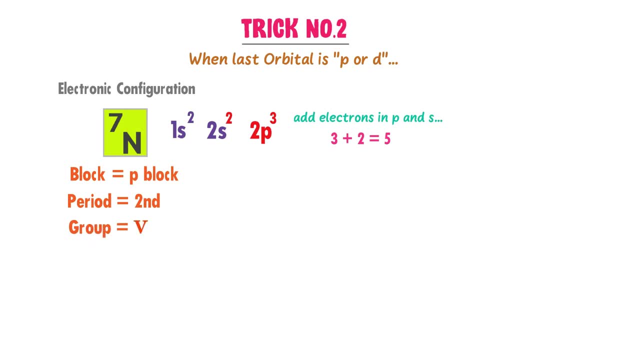 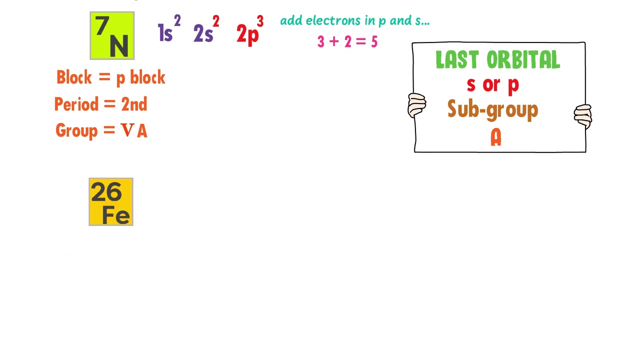 So nitrogen is in the fifth group. We also know that if the last orbital is SRP, its subgroup will always be A, So nitrogen is present in the fifth A group. Secondly, consider iron, and its atomic number is 26.. The electronic configuration of iron is 1s2,. 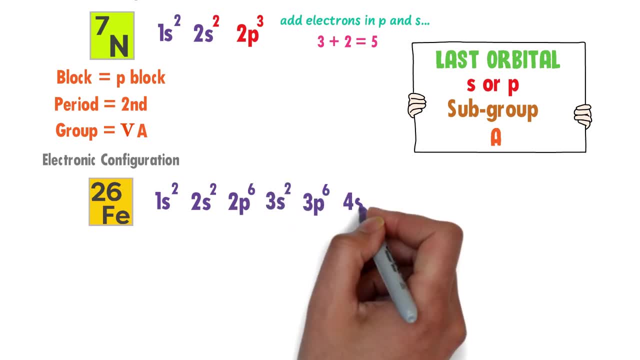 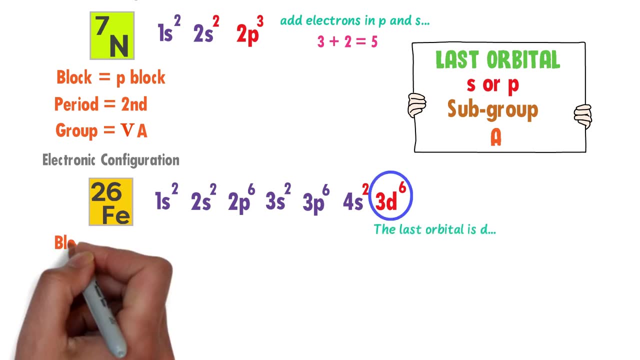 2s2,, 2p6,, 3s2,, 3p6,, 4s2, and 3d6.. The last electron of iron is in the d orbital, so iron is d block element. The highest principal quantum number of iron is 4,. 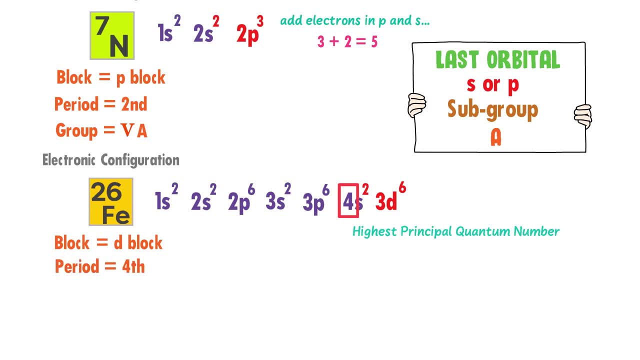 not 3, so iron is present in the fourth period. Now to find the group number of iron we have to add the number of electrons in the d and s orbitals. 6 plus 2 is equal to 8, so iron is present in the 8th group. Note it down that when last orbital is d or 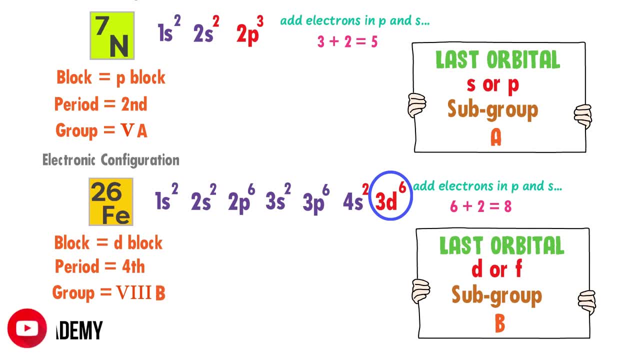 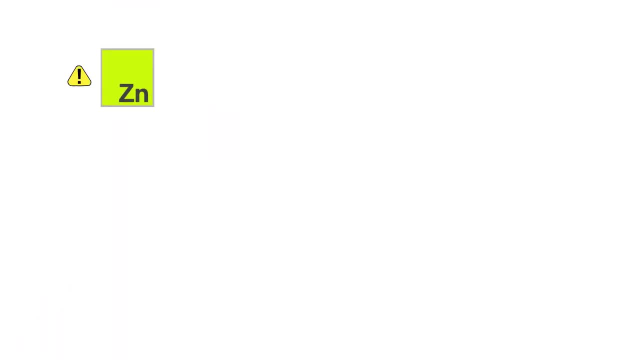 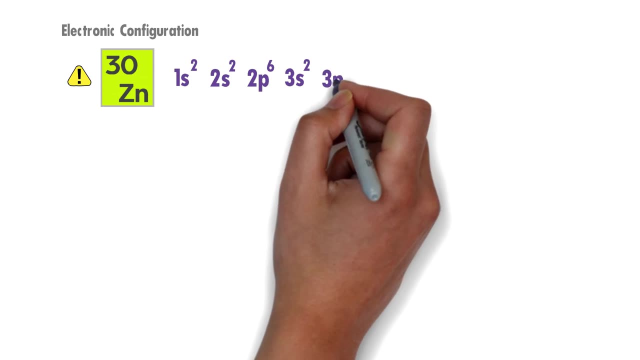 f, its subgroup will always be B, So the subgroup of iron is B. Now consider a special case like zinc, and its atomic number is 30.. The electronic configuration of zinc is 1s2,, 2p6,, 2s2, 3s2,, 3p6,, 4s2, and 3d10.. The last electrons of zinc are present in the d orbital, so zinc. 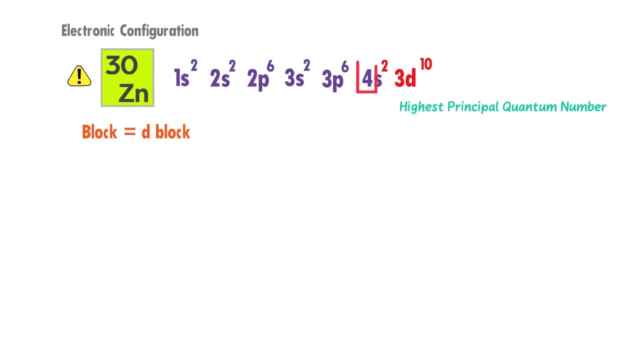 is d block element. The highest principal quantum number of zinc is 4, so zinc is present in the fourth period. Remember that d orbital is complete or filled because it can only hold 10 electrons. In such cases, do not add the number of electrons in the d orbital. 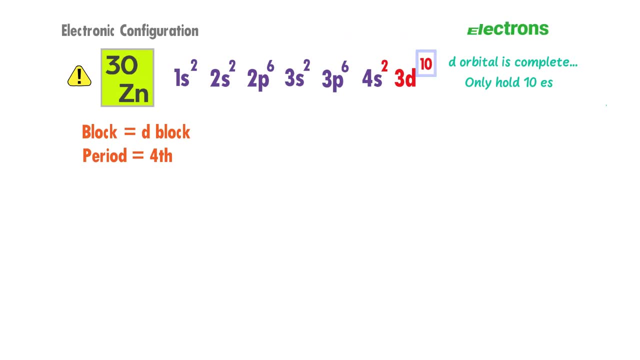 And add the electrons in d and s orbitals Directly, take the number of electrons in s orbital. There are two electrons in s orbital, so the group number of zinc is second. The last orbital of zinc is d, so the subgroup of zinc is B. thus zinc is present in the 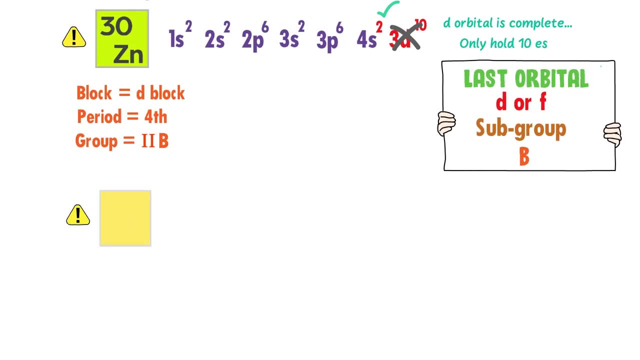 second B group. One another special case is nickel, and its atomic number is 28.. The electronic configuration of nickel is 1s2, 2p6,, 3s2,, 3s2, 3s2, and 3d10.. The electronic configuration. 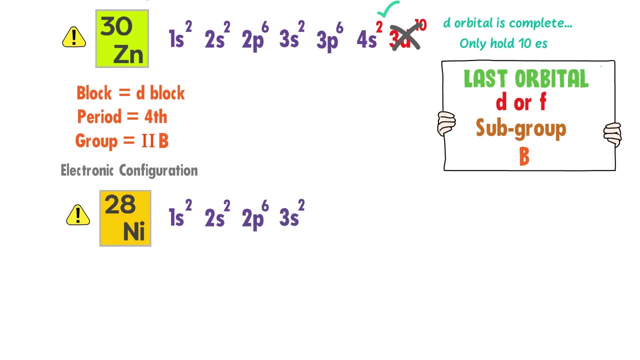 of nickel is 1s2,, 2p6,, 2s2,, 3s2,, 3s2, and 3d10.. The electronic configuration of nickel is 1s2,, 2s2,, 2p6,, 3s2,, 3p6,, 4s2, and 3d8.. The last electrons of nickel are in the d orbital. 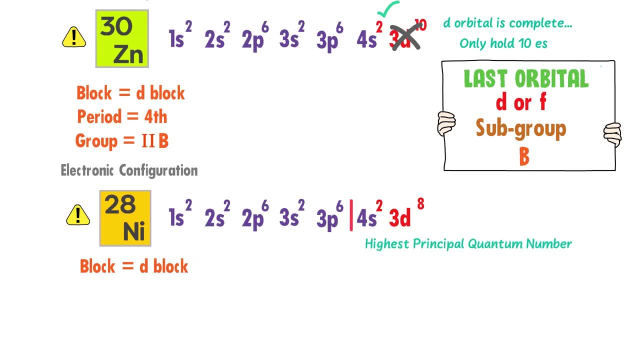 so it is d block element. The highest principal quantum number of nickel is 4, so the period of nickel is fourth. Now to find the group number, we add the electrons in d orbital and s orbital. Add plus 2 is equal to 10.. We know that the group number of electrons 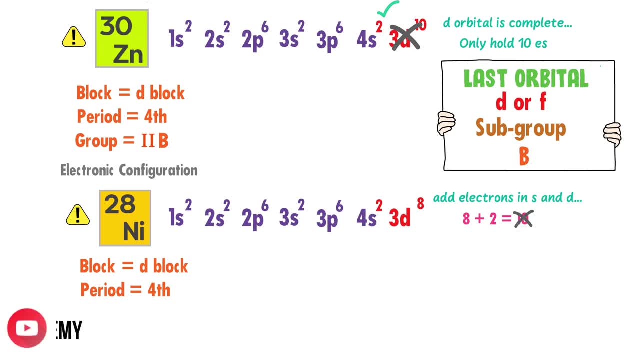 in d is equal to 10.. We know that there is no 10th group in the periodic table according to Riemann numerals, So whenever you get a number greater than 8 after adding electrons, remember that its group will always be 8.. Thus, the group number of nickel is 8.. The 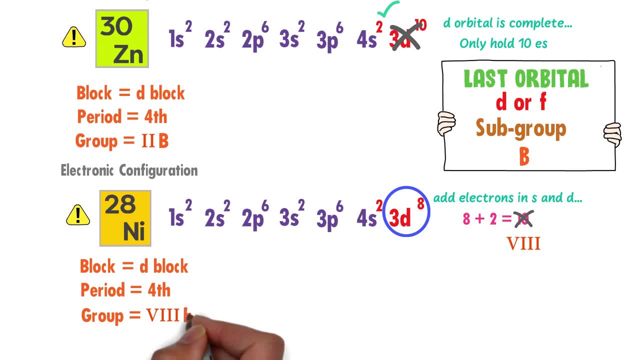 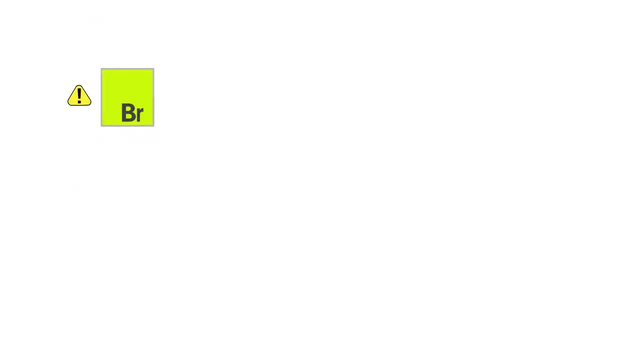 last orbital of nickel is d, so its subgroup is B. Thus nickel is present in 8th B group. The electronic configuration of nickel is 1s2,, 2s2,, 2p6,, 3s2,, 3p6,, 4s2,, 3d10, and 4p5. 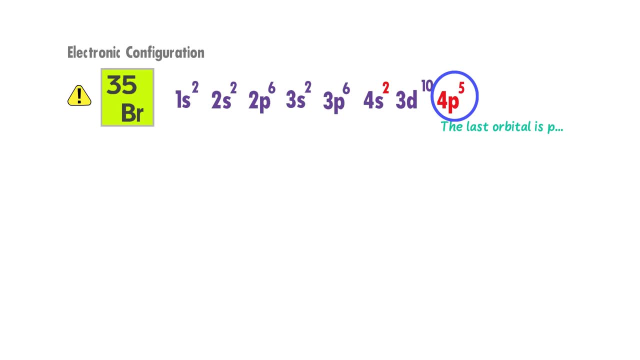 The last electrons of nickel are there in the p orbital, so nickel is a p block element. The highest principal quantum number of nickel is 4, so nickel is present in the 4th period. Now to find the group number we add the electrons in d orbital, so it is 2s2,, 2p6,, 3s2, and 3p6.